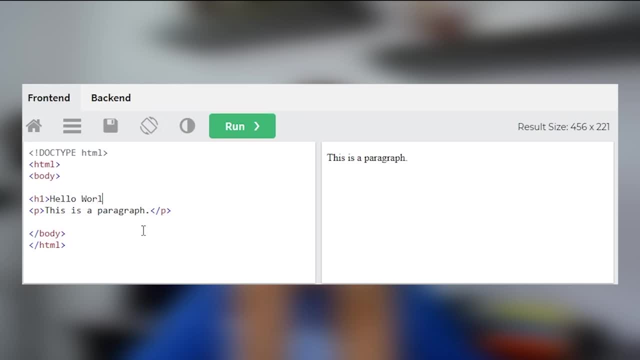 what you see on screen. So, for example, if you are looking to have a paragraph on screen, you would use the P tag. If you are looking to have an image on screen, you would use the IMG tag. These tags will show exactly what it is you are trying to. 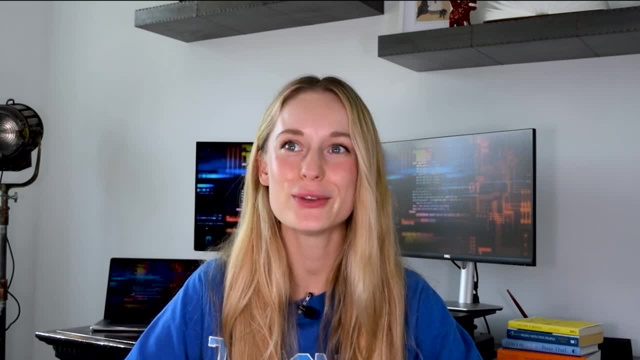 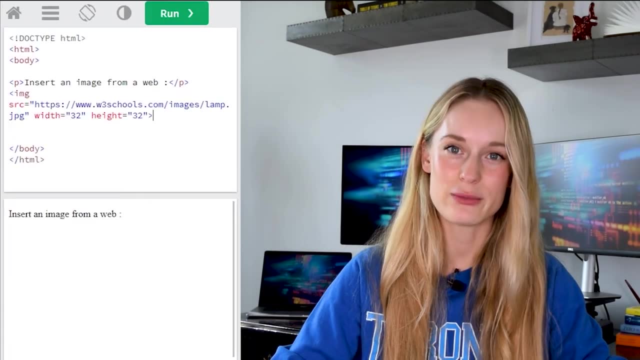 show to the user. I like to think of HTML as a way to have different instructions as to what to show to the user. So, for example, as I mentioned, the P tag to show paragraphs, the IMG to show images, and it's a really great way to think of HTML as a set of instructions. Websites would look pretty boring, though, if it was an HTML platform. If you think of HTML as a website with a lot of open space, you could build multiple websites with just one image, but what you do is you create a database of different attempts to understand the information. 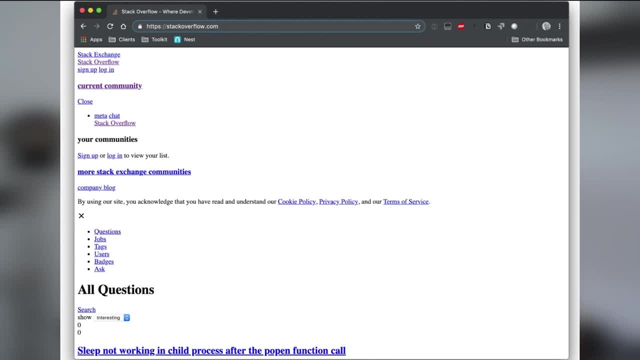 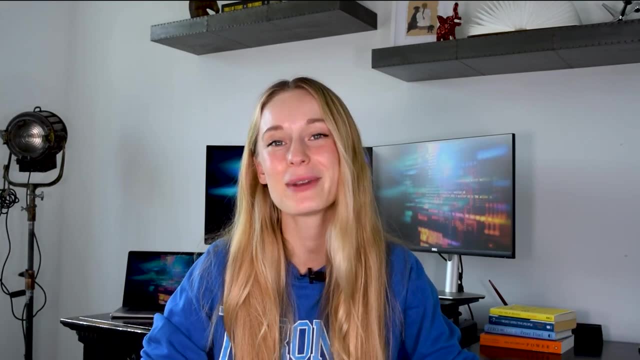 wasn't for the help of CSS, As you can see, this would be a website without any CSS. It's boring, it's plain. I mean, who would really wanna use any websites? And that's where we go to CSS, While HTML is the markup language. 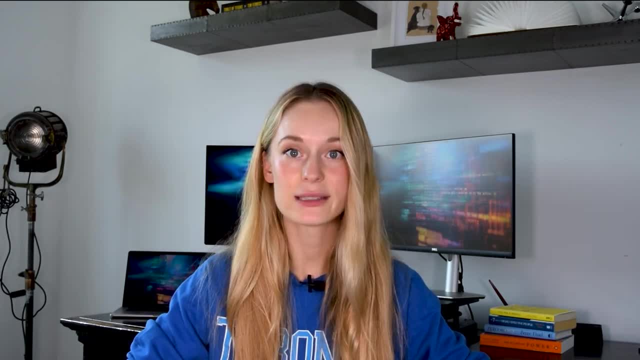 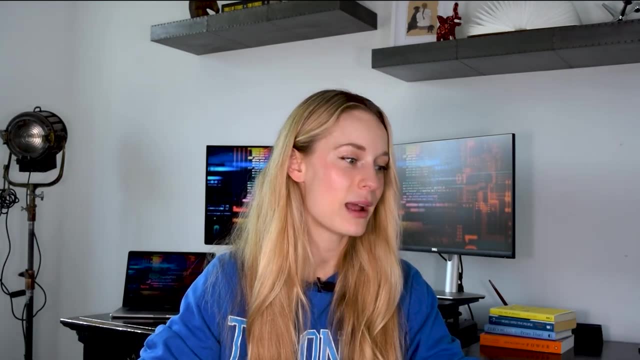 CSS you can think of as the design language. CSS stands for cascading style sheets And there are many different versions of CSS, many different takes on it, but at its core, CSS is used to make a website look good. Sounds simple, right. 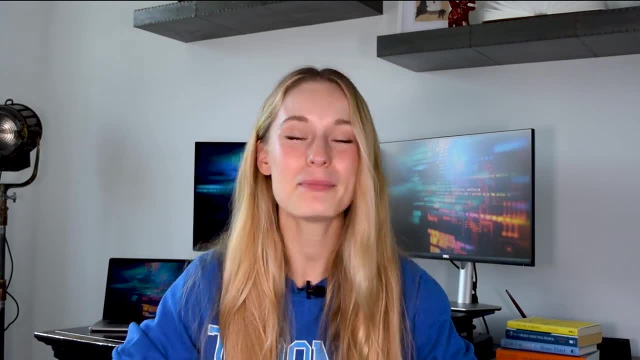 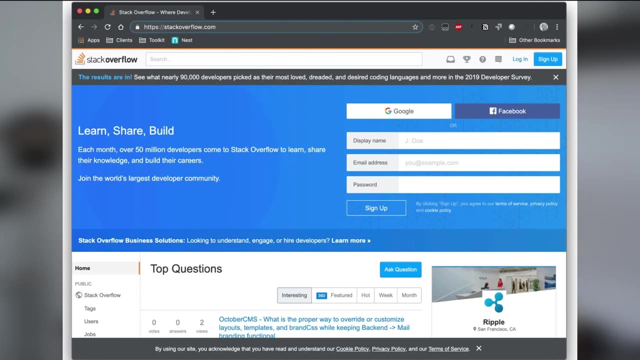 Why complicate things? It does get complicated the further you get into it, but at its core, that's what it does. I'm going to show you a website here that has CSS. As you can see, it's a no-brainer. 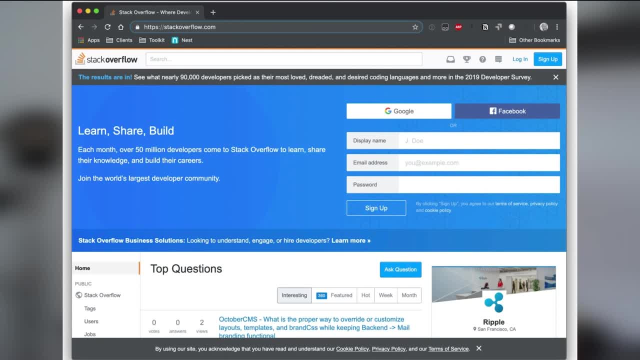 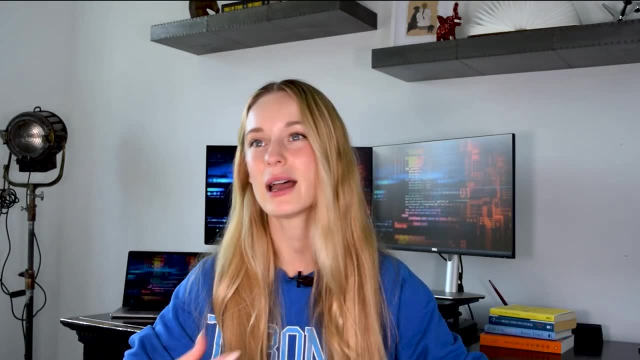 It makes things just instantly look so much better. I think as humans, we are so visual, so CSS is so important. I often hear people say front-end is boring, or designers or front-end people: they have such a boring job, which is completely not true. 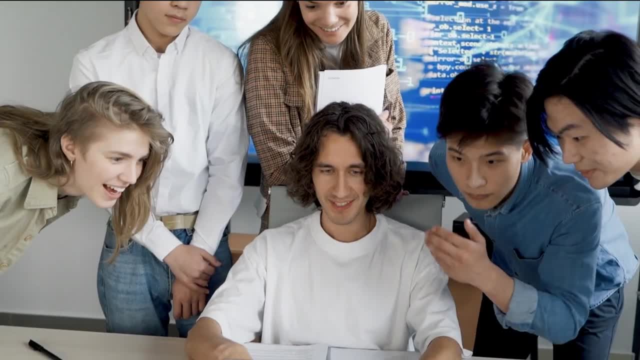 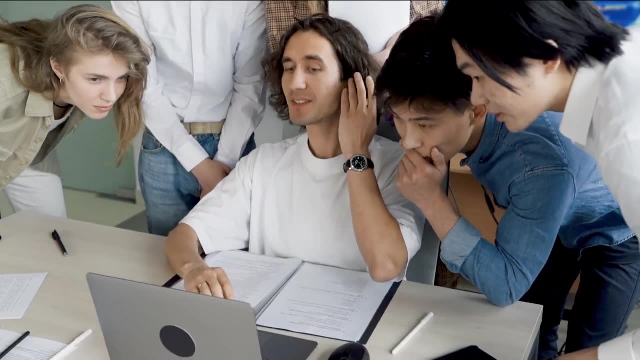 I think it's just because back-end is having a moment, but in reality, these people who focus on front-end or design, they have such an important job to ensure that when a user goes to a website, for example, they actually stay there right away. 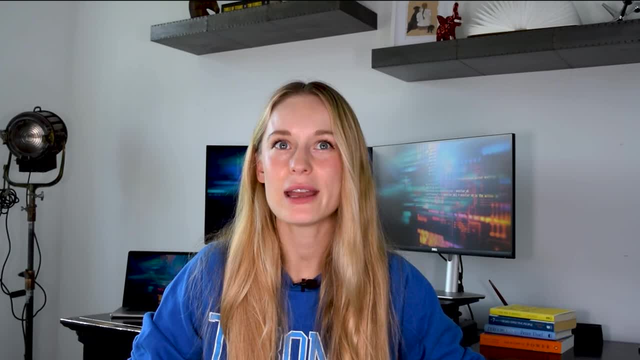 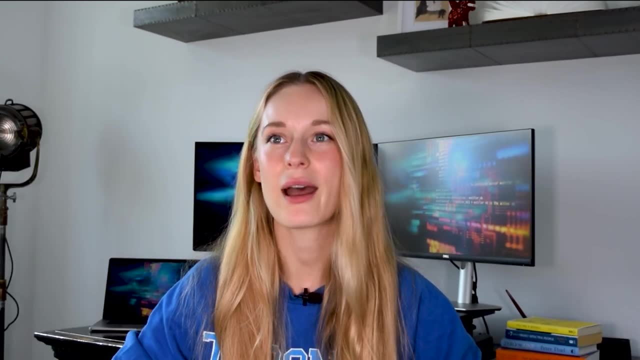 because of what they see visually. When you think CSS, think of it as a list of rules that you can assign properties to different HTML tags. You can make each tag look unique, have different styles, depending on what it is Before CSS. this was. I'll show you on screen. 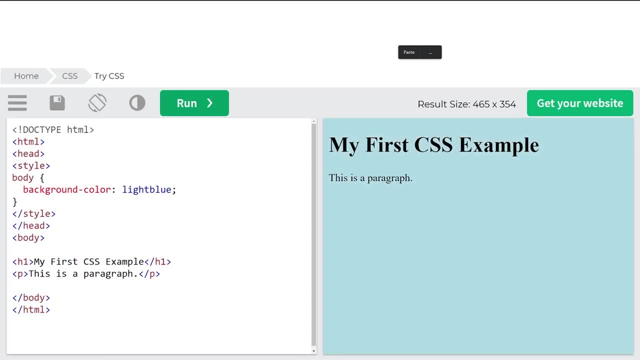 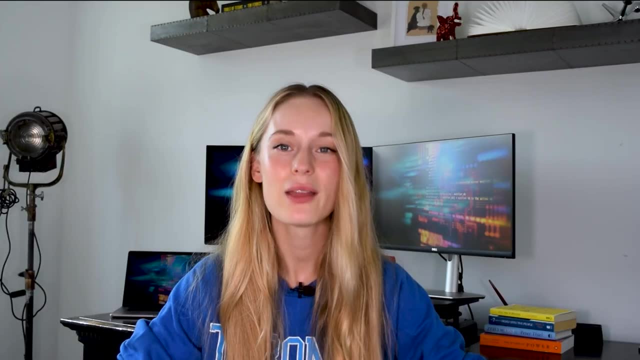 how to write styles. As you can see, it would get very inefficient as it continued to get longer and longer with more styles, writing it directly in line in the HTML tags. That's why CSS is so amazing to have its own file where you can put all the different styles into it. Nowadays there are so many different CSS frameworks that you can use that really help speed up the process when you are designing or developing a website and the look of it. Some include Tailwind, Bootstrap, Pure CSS, Foundation CSS. I would say Tailwind and Bootstrap right now. 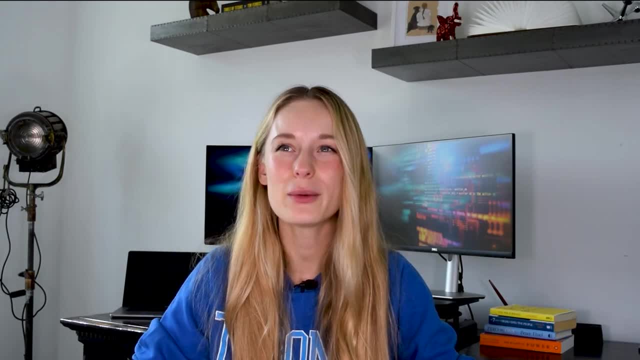 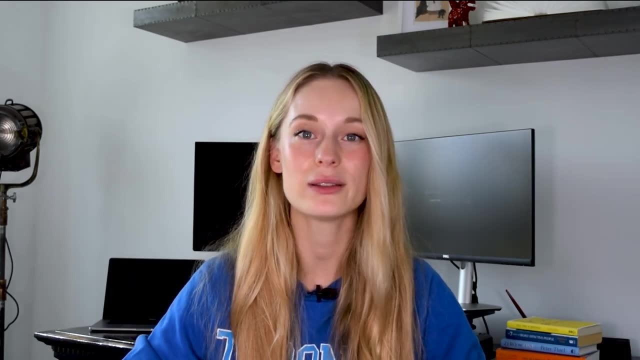 are definitely the most popular ones. I've used Tailwind a little bit, Bootstrap a ton in the past, and at this point it's literally between their documentation and the community online. it makes it very easy to start using. Okay, so if I put this website on screen here, 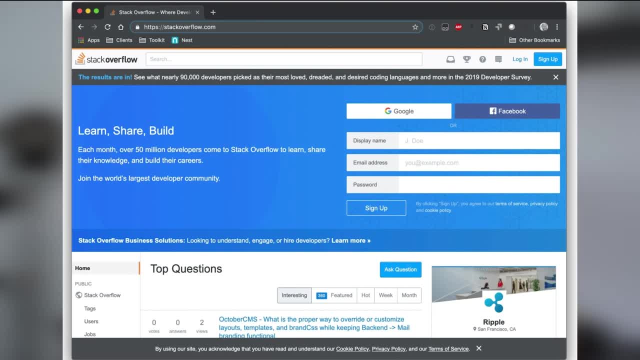 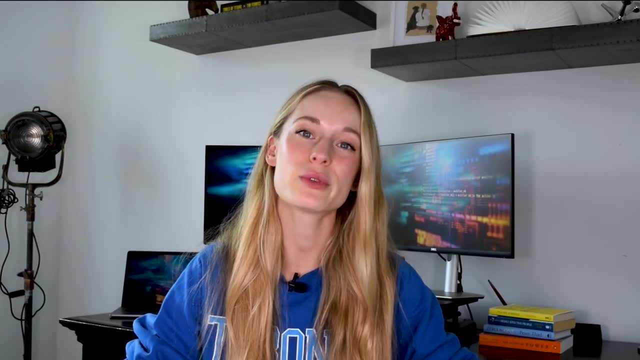 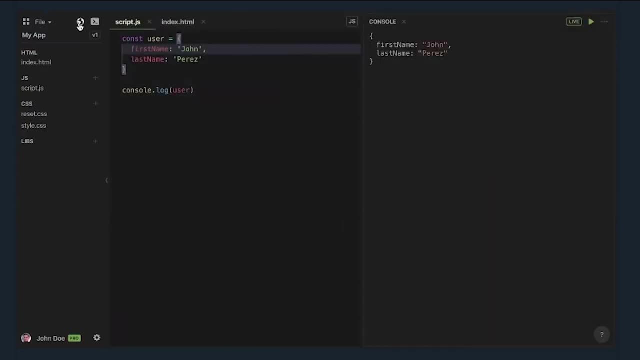 now that we have HTML and CSS, you can see that it looks fine. What really are you missing? Probably nothing, until you start interacting with it, And that's where JavaScript comes in. JavaScript, essentially, is a programming language that is used to help with the user interacting. 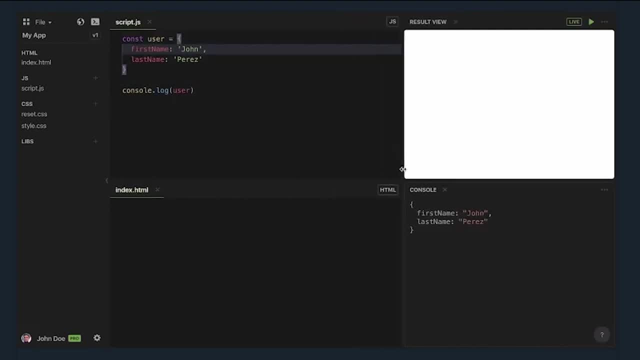 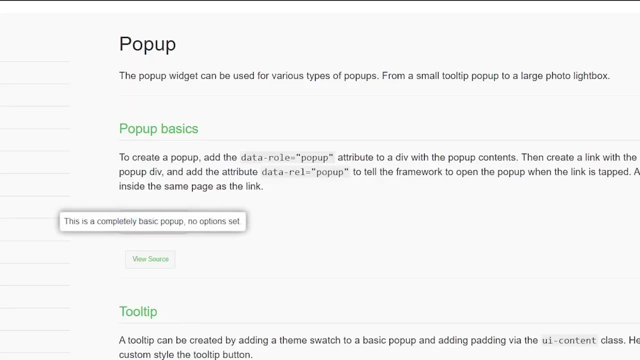 with the website. So what I mean by that is actually I'm gonna put up on screen here. when you interact with the website, you will get a response back from the website. This might be a pop-up, this might be notifications and animation. 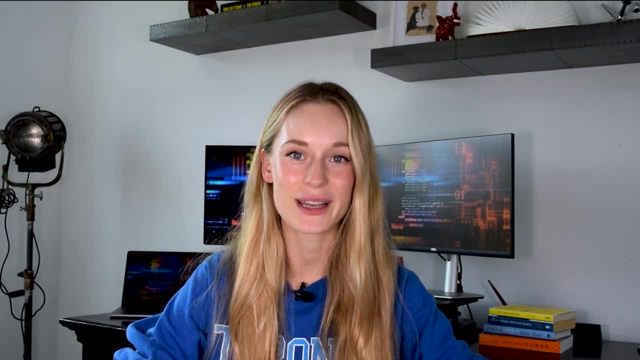 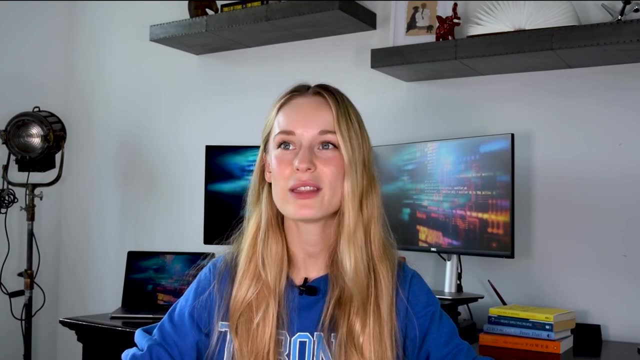 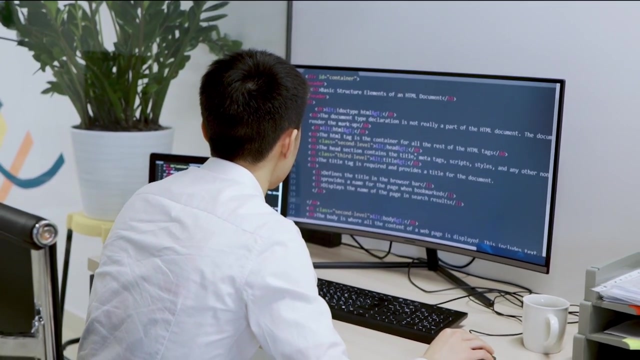 and so much more. Most dynamic behavior you see on websites is thanks to JavaScript. JavaScript has many different frameworks and libraries that can be used And if you're learning JavaScript, you will be able to use them with it. But I always say if you are learning JavaScript. 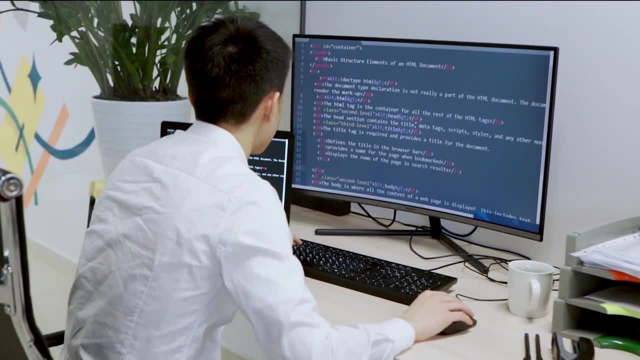 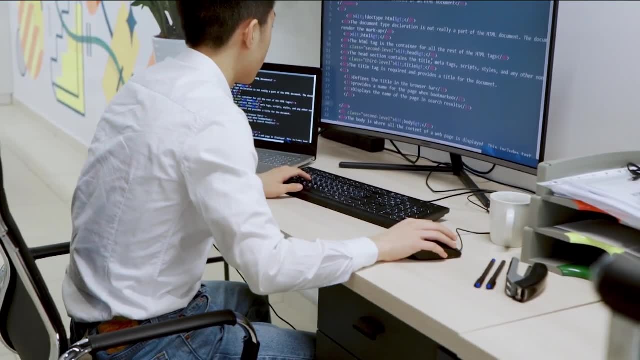 start with vanilla JavaScript. JavaScript is widely used across the web and now is used not only both in the front-end side of things and also, to now, it's used in the backend with Node and Express. For the purpose of this video, though, we are going to talk mainly about. 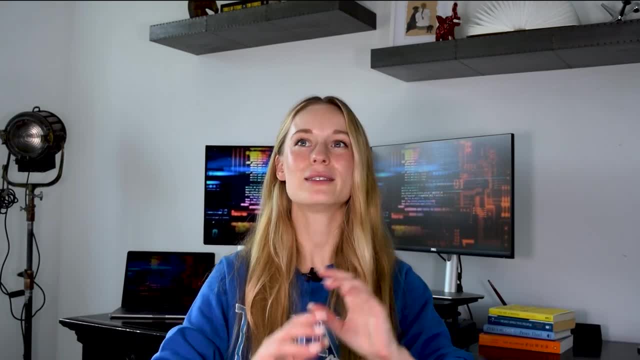 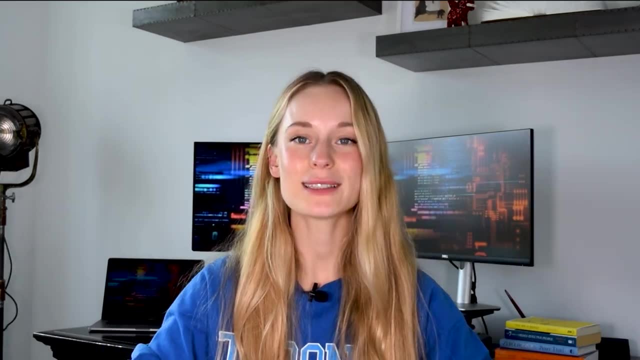 the front-end use with JavaScript, When you think JavaScript it's not necessary to add to make a website. It's a possibility to the website and make it more exciting for the user. So next time you think JavaScript, essentially just think of it does something. 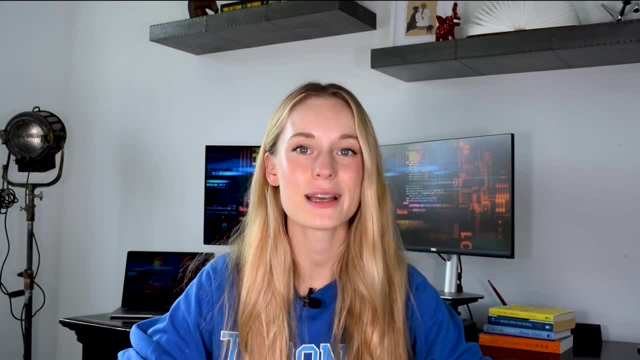 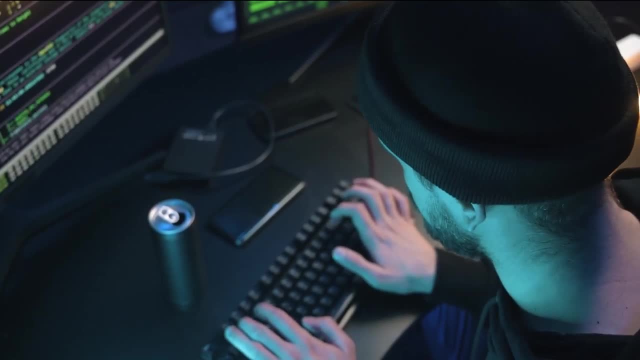 it tells the computer to do something. Here are a few more things that JavaScript is used for. You can use JavaScript to add interactivity to websites if you want to make a website more than a static page, as we spoke about. Also, you can use JavaScript to develop mobile applications.